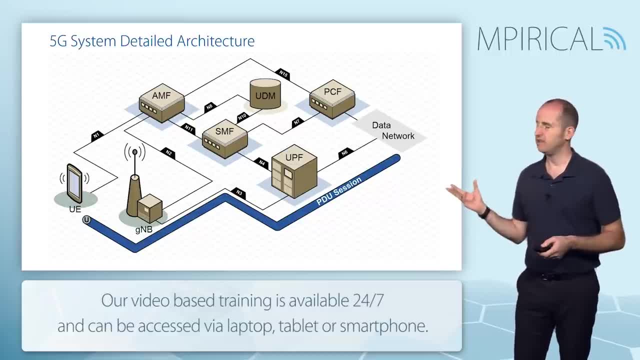 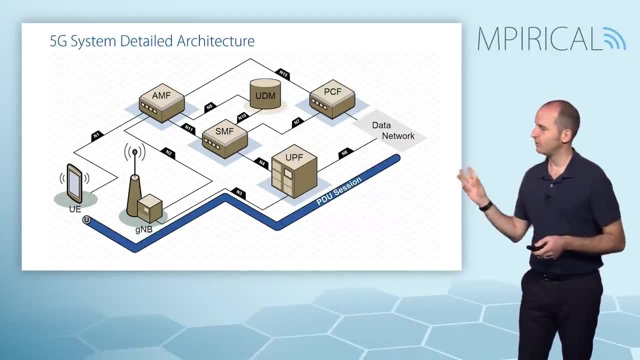 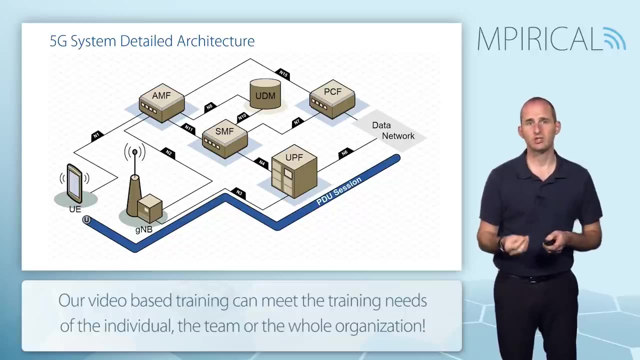 plane connectivity and that user plane connectivity in 5G is called a PDU session, a protocol data unit session, and you can see it runs from the mobile or from the device through the GNB to the UPF, the user plane function, and then on to the data network. So traditionally in LTE, for example, it 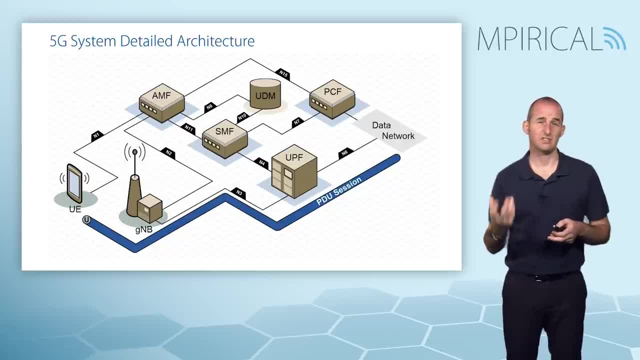 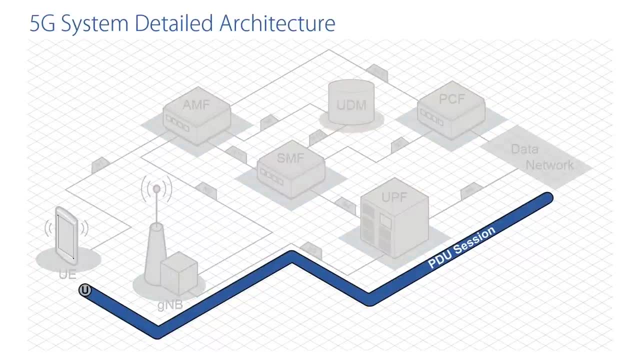 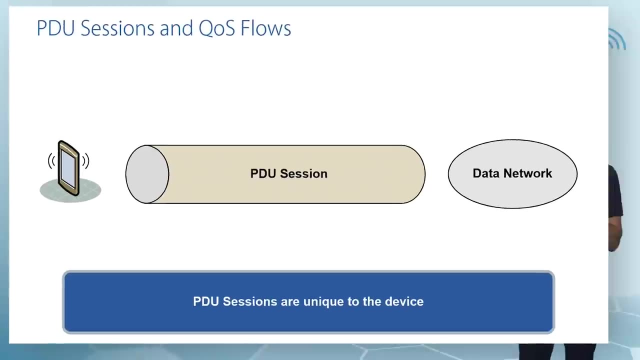 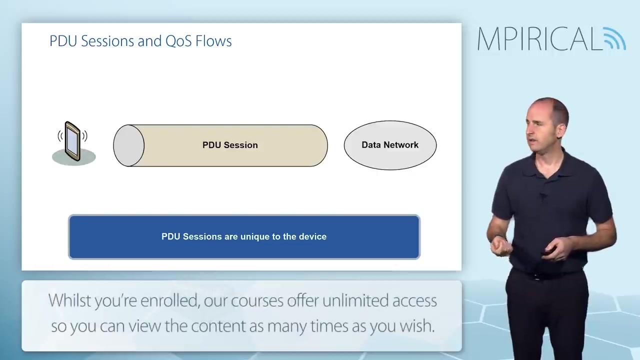 is called the data network. In 5G it's the data network, but this is going to be the internet or perhaps the IMS or a corporate LAN of some description, So no other devices in the network will be using the connectivity associated with this particular PDU session. Now, in order to provide QoS, 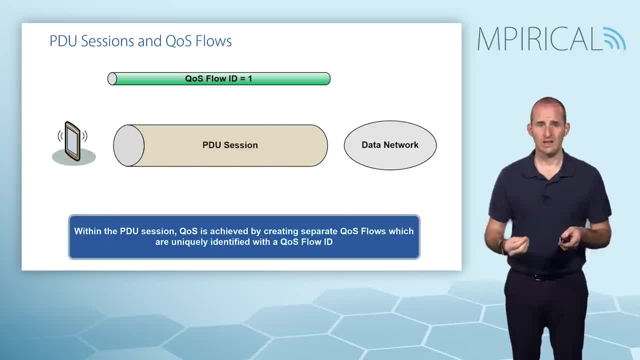 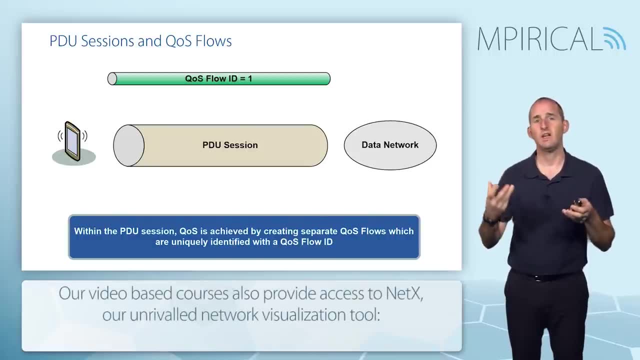 we have what are called QoS flows. Now, a QoS flow is effectively a flow of user plane traffic which will be receiving a particular level of quality of service. Now, because we might have traffic with different QoS requirements. what that might mean is within the PDU session. 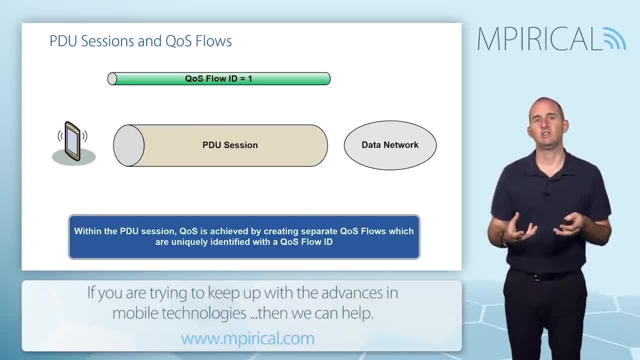 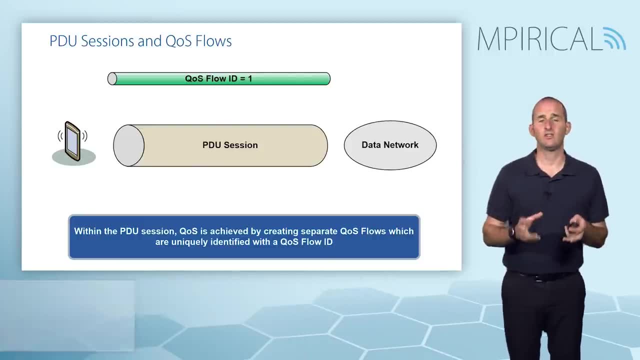 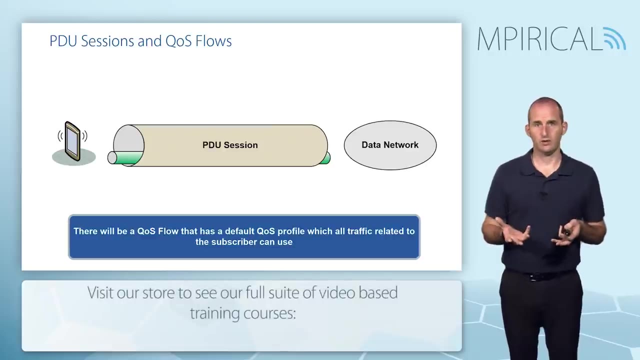 there are several QoS flows actually in operation. To distinguish between them, each QoS flow has a QoS flow ID and to begin with, we will have, if you like, a default QoS flow and this default QoS flow. it will have a particular level of quality of service. 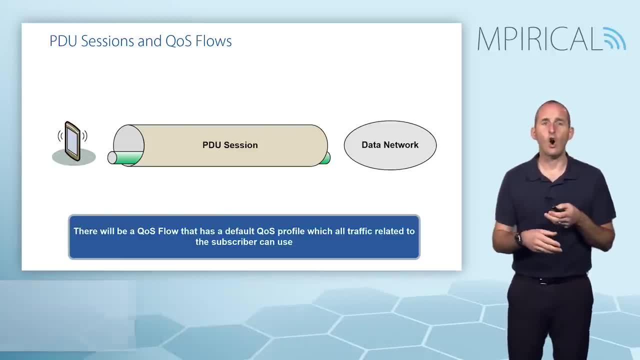 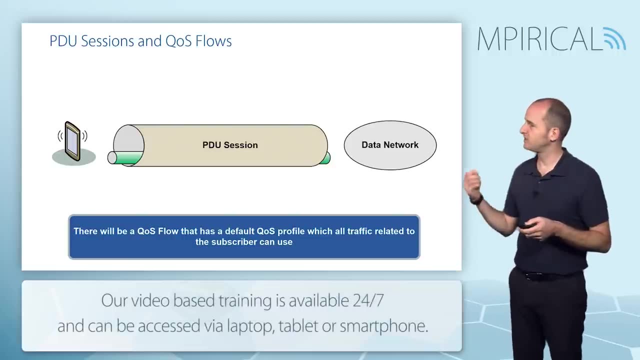 but it won't have any kind of packet filtering on it, so all packets can potentially go down this QoS flow if needed. However, as soon as we start adding additional QoS flows with different QoS requirements and different QoS levels, then we will start filtering which. 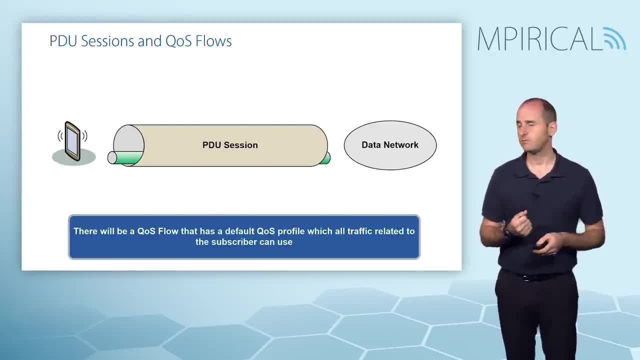 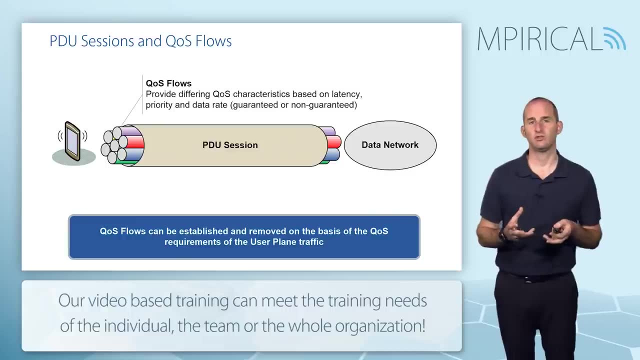 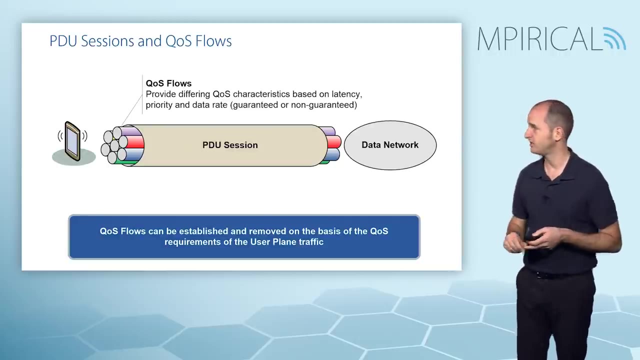 traffic can actually go down these barriers. So you can see that, in actual fact, within a PDU session, we could have several QoS flows in existence, and you can see that the kind of QoS flow characteristics we see for quality of service are things like latency, priority. 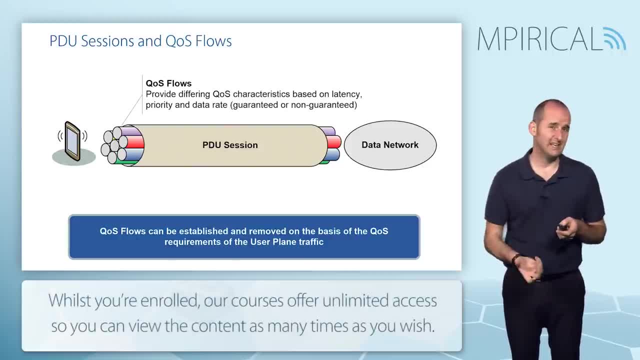 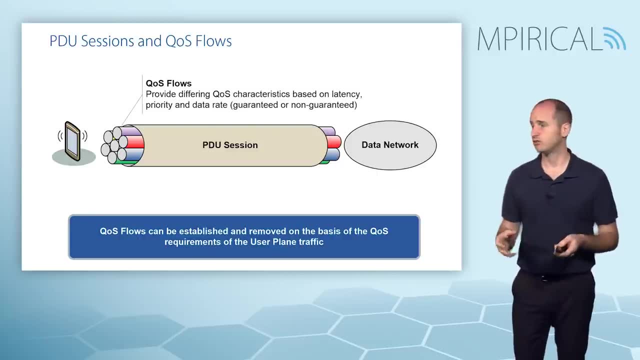 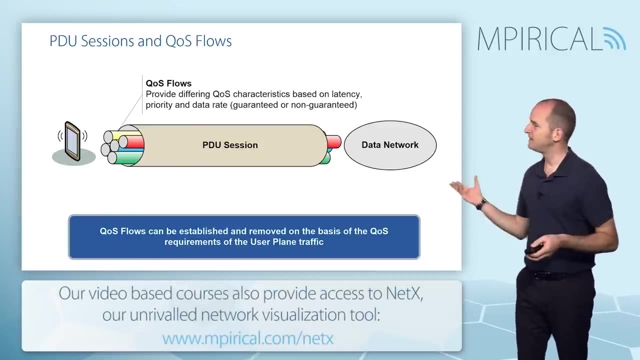 and whether or not this particular QoS flow is guaranteed bitrate or non-guaranteed bitrate and, as appropriate, these flows can be transient so we can actually remove flows if necessary. Now, being realistic about this: if the data network was the Internet, for example, then we typically only need one QoS flow. that would be the default. 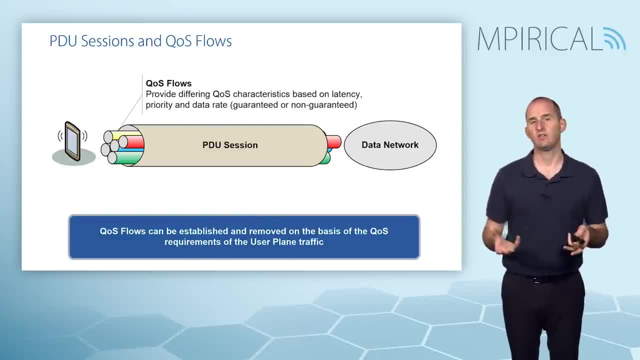 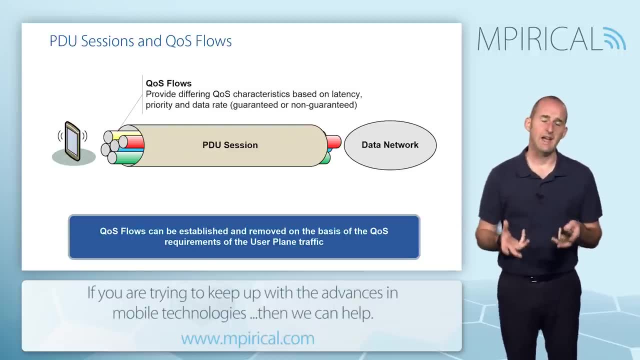 flow, and that would be a best-efficient QoS flow effort: QoS flow. If, however, this is maybe 5G voice services and the data network is the IMS, then we could have a QoS flow that's carrying the signaling associated with voice. 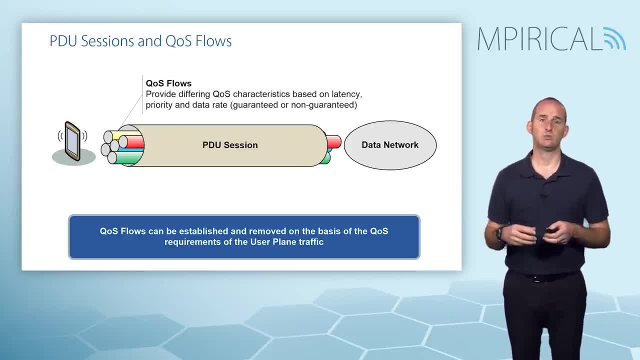 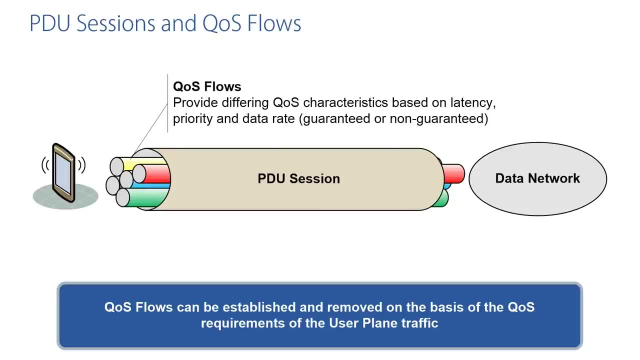 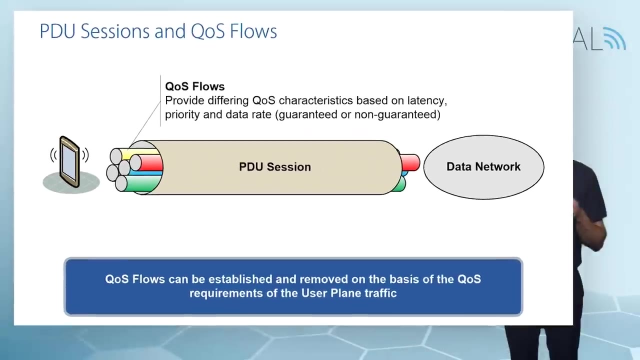 and then we'd have a separate QoS flow that's carrying the actual voice packets themselves And, as traffic traverses the QoS flow, it actually has a QoS flow ID added to the traffic protocol stack, so we know exactly which flows a particular piece of data should go. 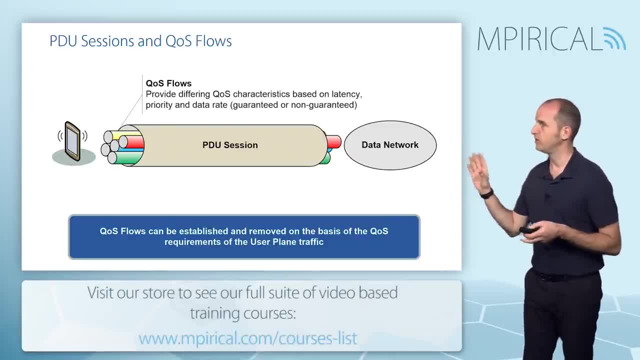 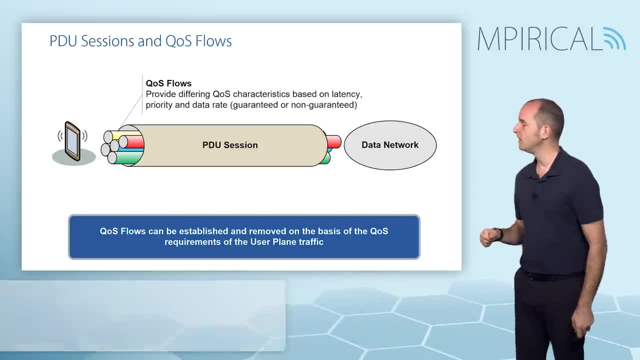 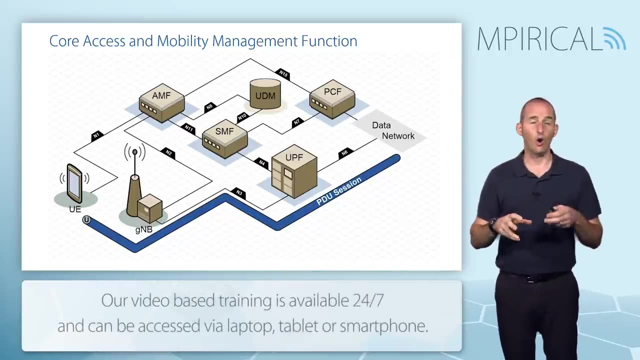 down, But certainly to have lots and lots of QoS flows. well, we'd really need to consider what scenario would actually require that. As we move on to our actual architecture, though, we'll look at each of these various elements in turn now, all fundamentally designed to keep that PDU session active for the subscriber. 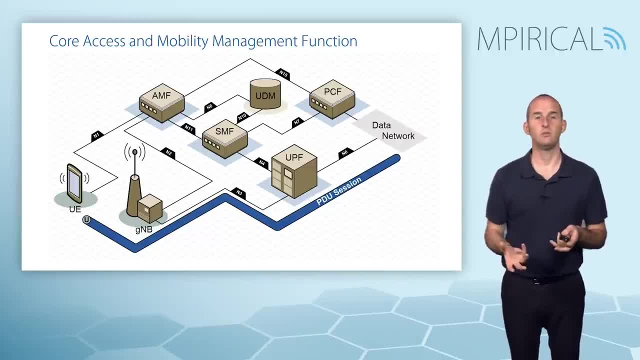 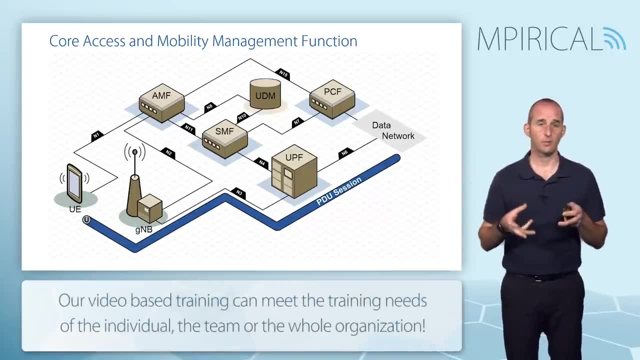 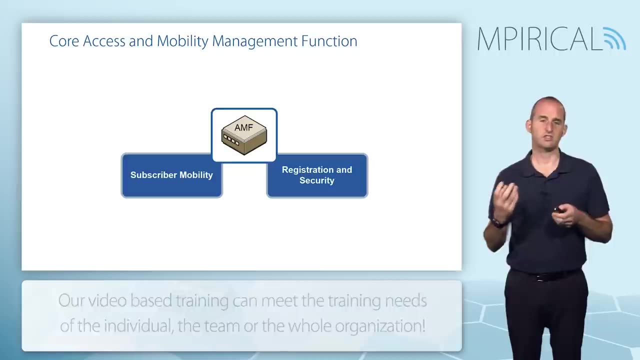 and ensure that flow. Fundamentally, the PDU session follows them as the subscriber moves around the network. So, to begin with, the first element that we're going to consider that we find in the core network is the core access and mobility management function, And this has got a similar role. 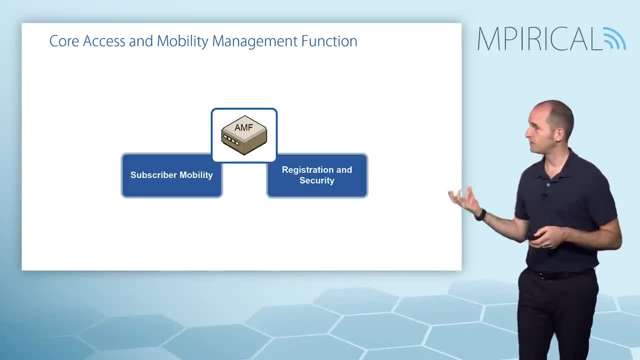 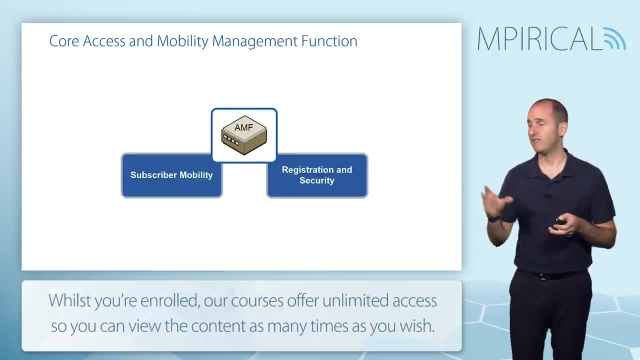 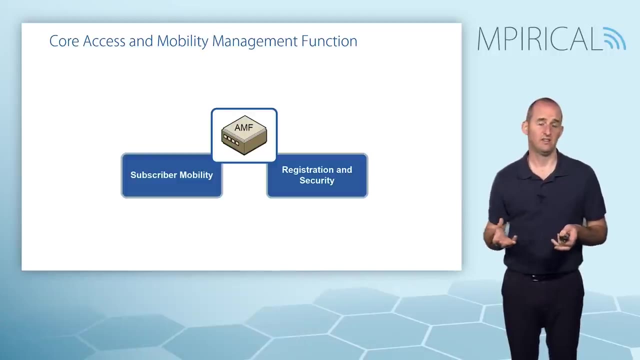 to the MME in LTE, whereby it looks after mobility management. So, in terms of subscriber mobility, we consider the fact that this AMF will always know either the tracking area that the subscriber is in or the potential cell that they're in. 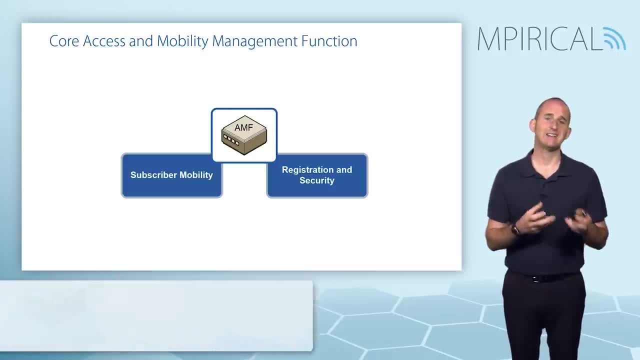 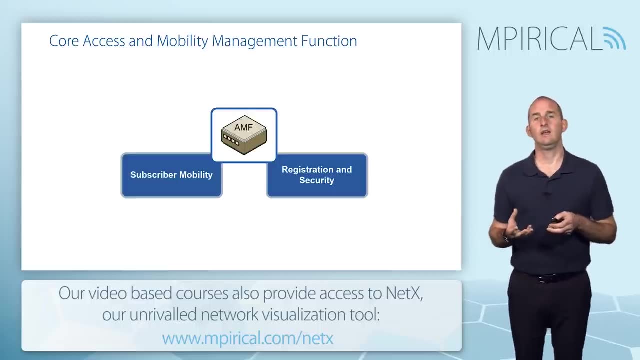 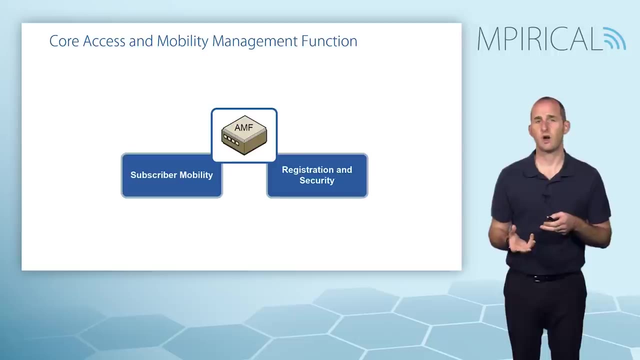 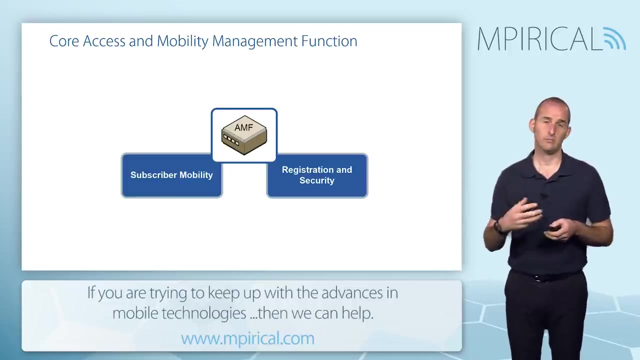 And it really depends on whether the subscriber is idle or connected respectively. The AMF, though, also plays a key role in security and registration, So it's the AMF that will be liaising with various other subscriber databases to ensure that the subscriber is allowed on the network in the first instance, and the AMF will play 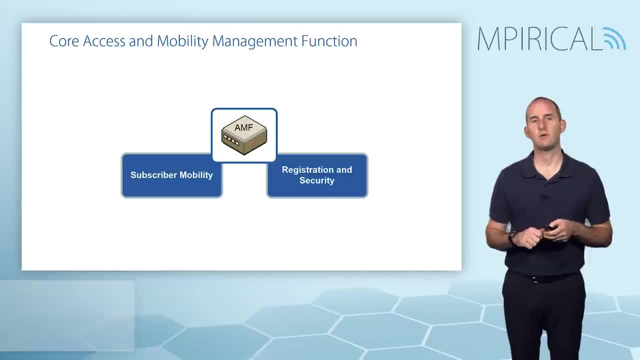 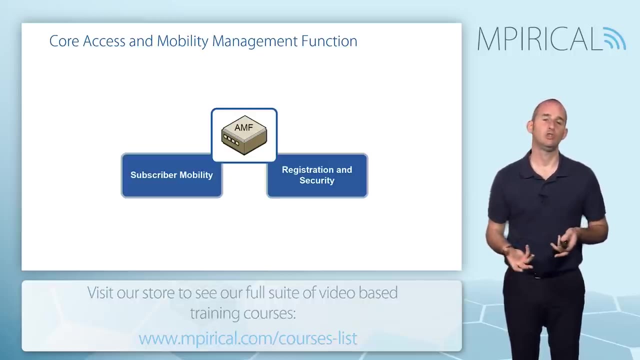 a key role in belonging and accessing the network, role in authenticating that subscriber within the network. Finally, the AMF will also provide the device with a temporary identity which you can use whenever it signals the network. That temporary ID is also used in paging as well. 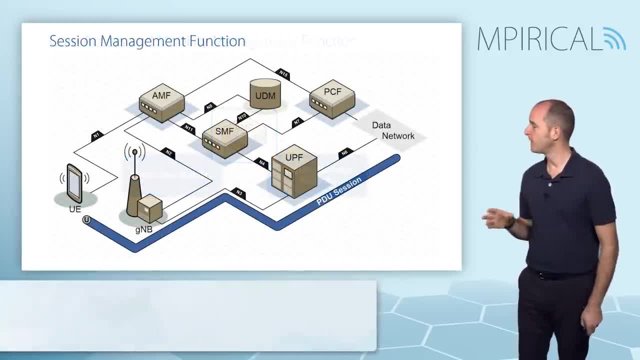 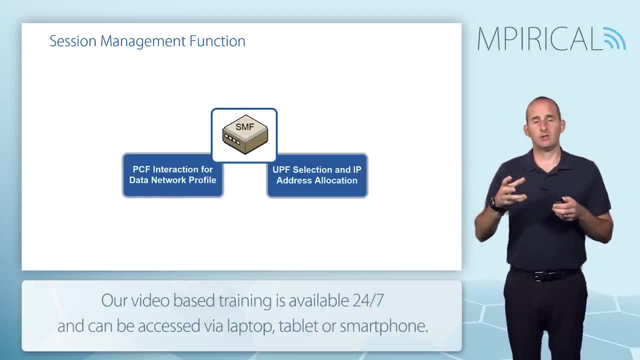 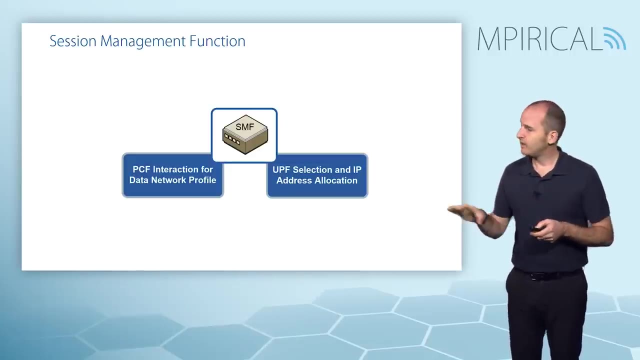 So that's the core access and mobility management function. Moving back to our architecture, the next element is the session management function. So traditionally in LTE it would be the MME that does mobility management and session management. We can see that in 5G that functionality has actually been split. 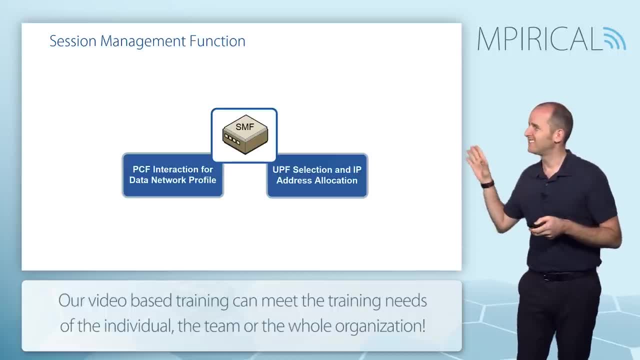 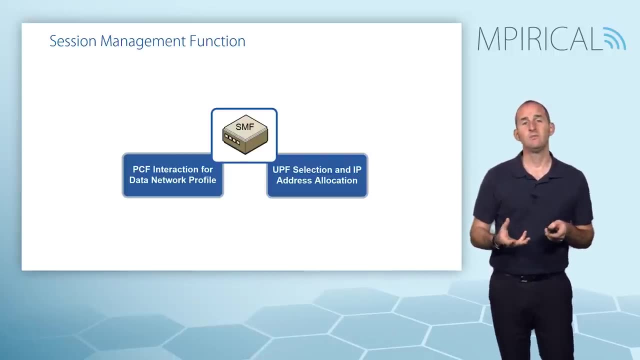 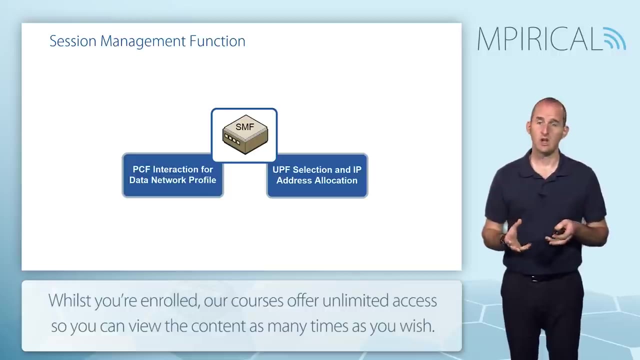 So it's the AMF that does mobility management and here the session management function does session management. So what we're effectively talking about here is the establishment and the modification and the teardown of our PDU sessions. So the SMF is directly involved in that and as part of that it will be routinely liaising. 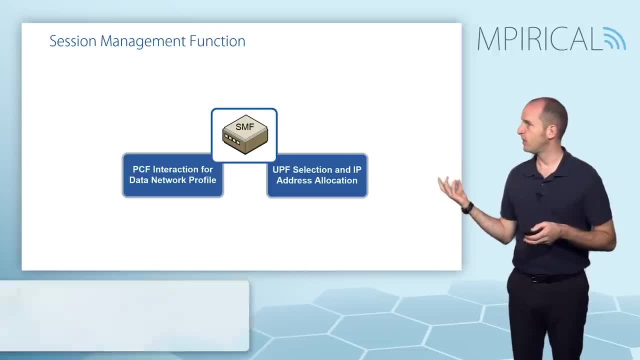 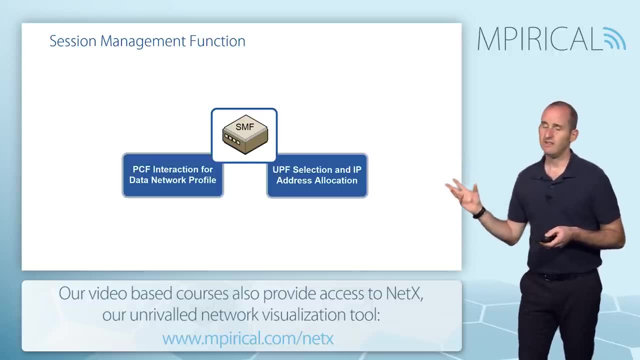 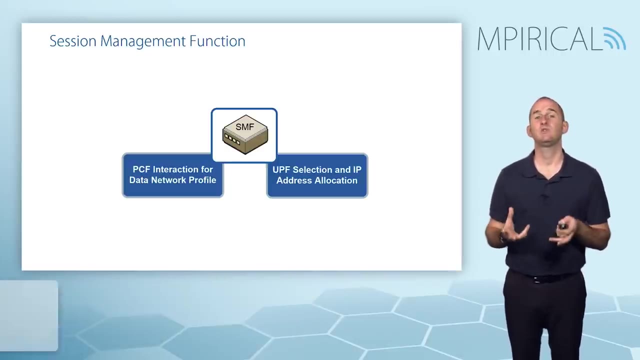 with the policy control function to determine whether or not a particular user data session is allowed to go ahead. Not only that, the session management function is directly involved with the establishment of the actual PDU session connectivity, So that pipe that we draw on our diagram which is representative of the PDU session. 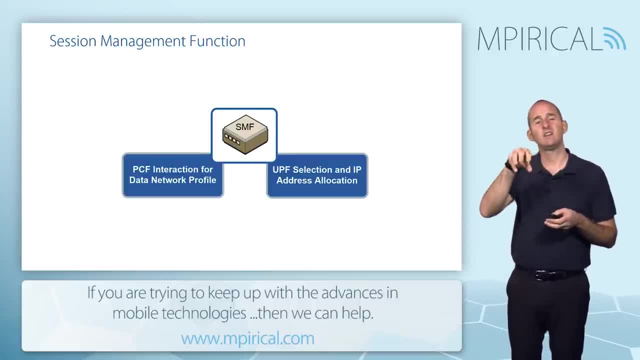 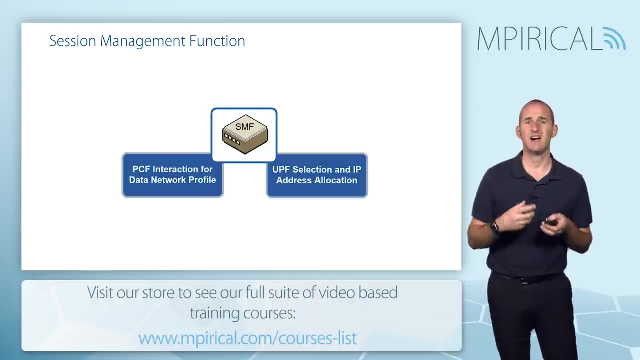 is actually a series of separate connections that must be set up in the network. Now those connections run through the user plane function and it's the job of the SMF to choose which UPF. And also, if the data session is IP based, the SMF will also be allocating an IPv4 or 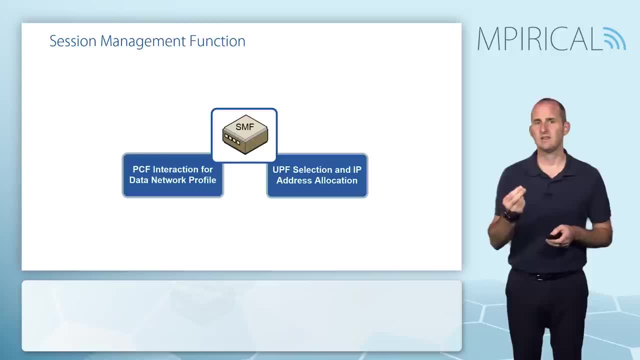 an IPv6 address. Now I did say if, because PDU sessions can actually be based on purely IP. It's not just purely Ethernet or even unstructured data in 5G, It's not all about IP like it was in LTE. 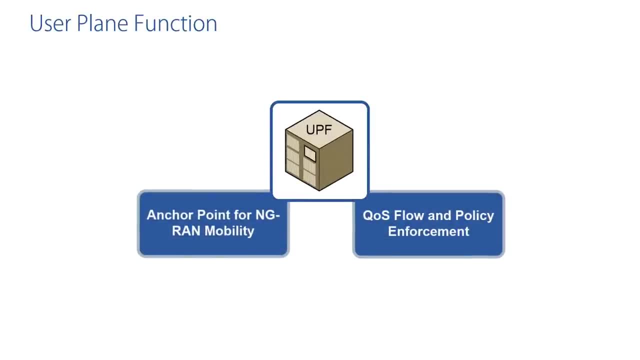 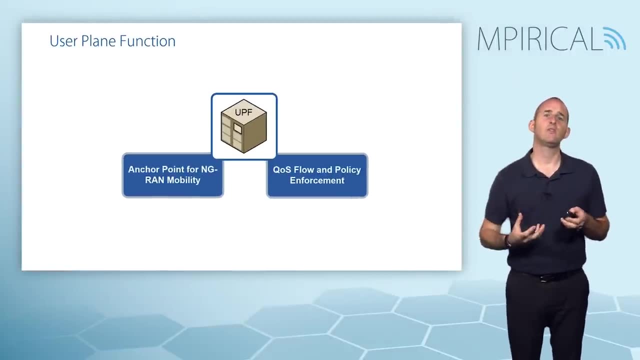 As we move through the network, we've got our user plane function- We've already started to touch on this- And, as you can see, it is an anchor point for NG-RAN mobility. So as I move around the radio access network, I will move from one GNB to another. 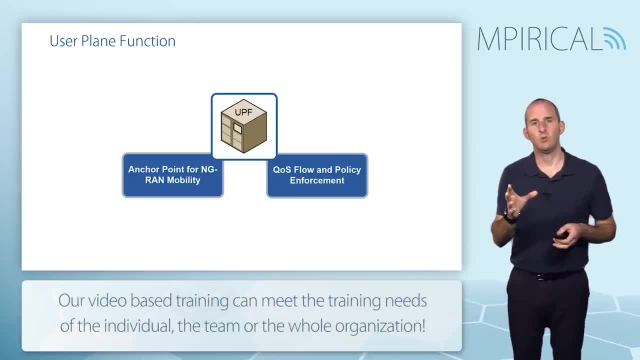 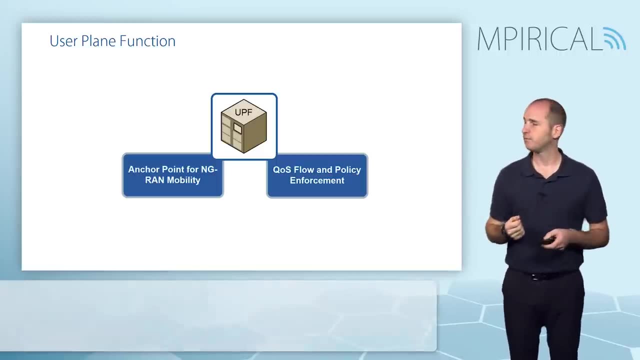 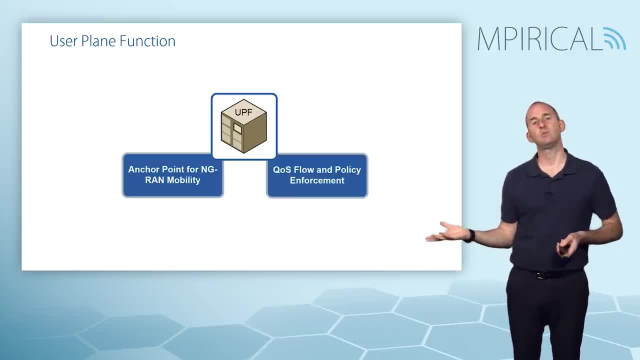 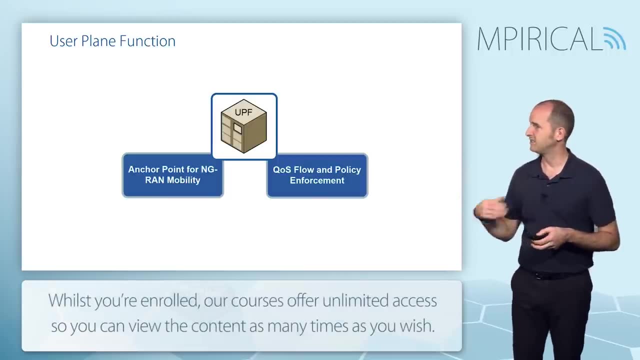 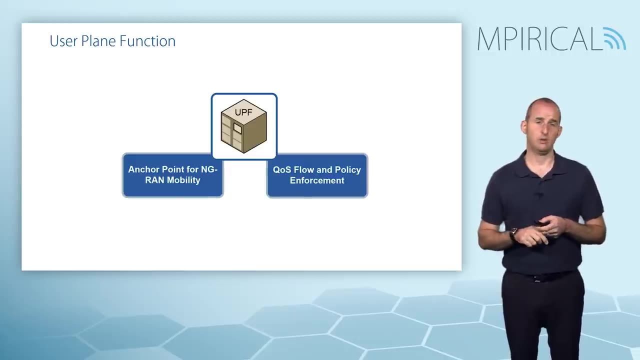 And because the UPF is directly sat on the user plane, it's an ideal point to enforce quality of service. That's, ensuring that the right data is sent down, the correct QoS flow And also implementing policy as appropriate, And that could be throttling of data, for example. 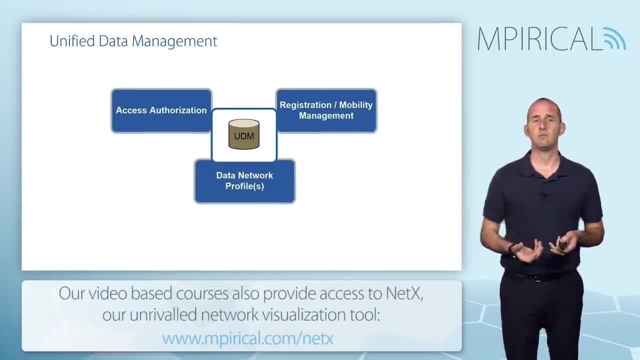 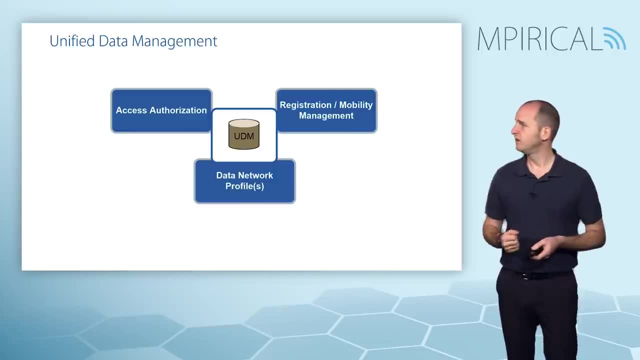 As we move through the network. the next element that we have to look at is the network traffic have is the UDM, and this is unified data management. in effect, it's a central repository of subscriber information, directly involved with access authorization, because it will be holding security keys. it's also involved in 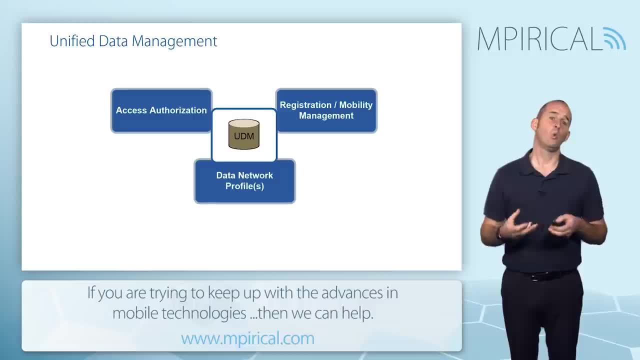 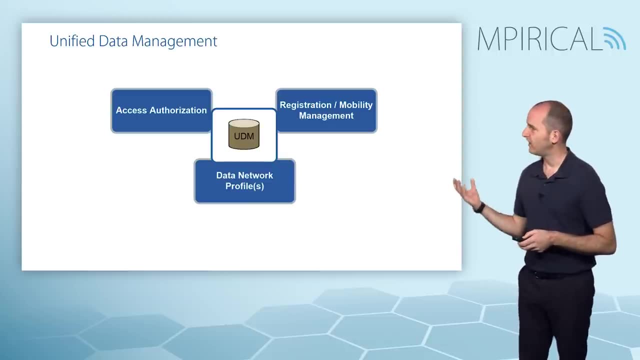 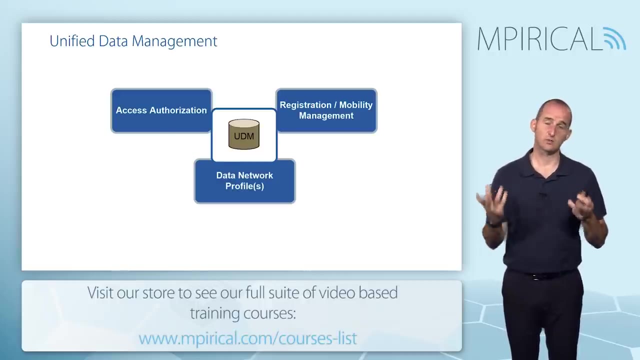 registration and mobility management, because it will be tracking where our subscriber is attached to, in terms of which AMF our subscribers being allocated, and then, finally, it will contain the data network profile or profiles. it effectively contains the subscriber profile, telling entities like the AMF and the SMF exactly what our subscriber is and is not allowed to. 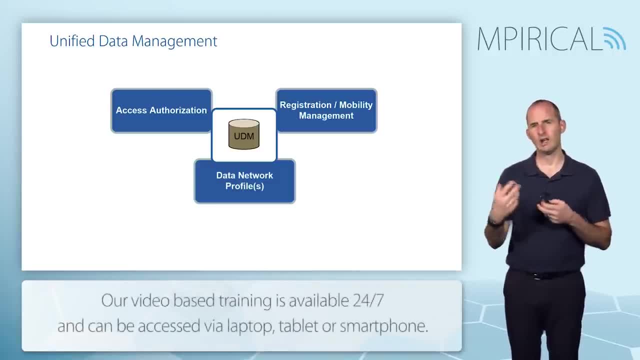 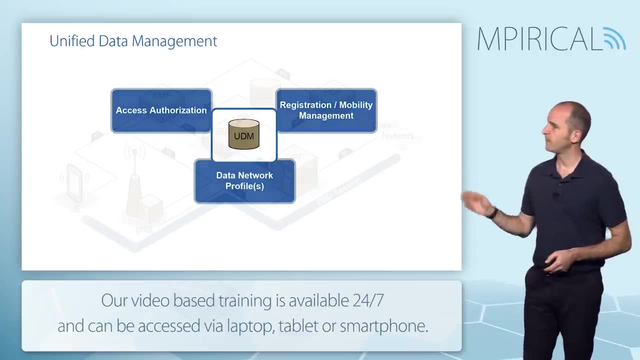 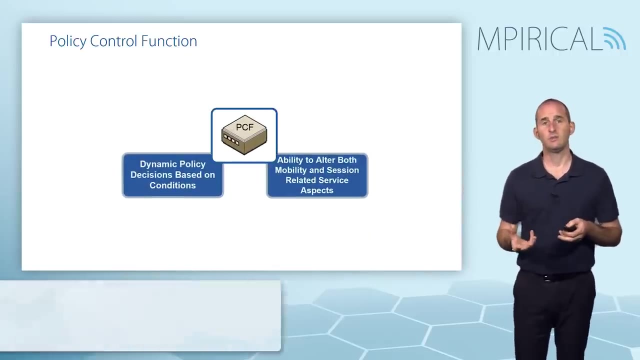 do, which data networks they can connect to and what kind of QS profile they can expect to be granted when they do connect to those data networks. next in line, and finally, is the PCF. and the PCF is there to implement policy control approach, policy control function. and when we talk about the PCF and implementing 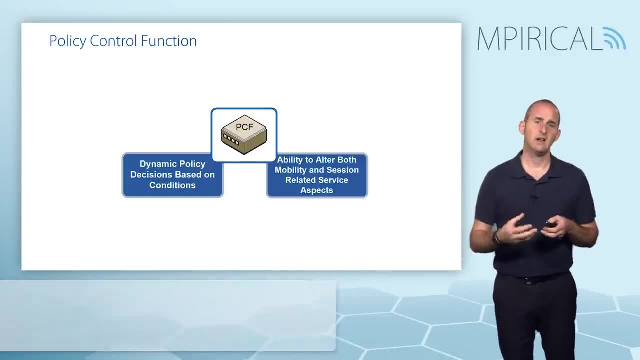 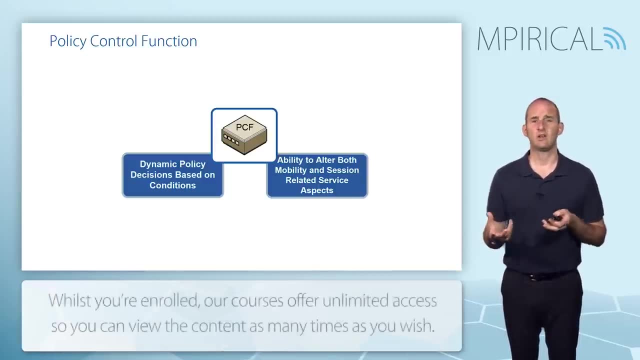 policy control. it's all on a dynamic basis now. the dynamic policy decisions are based on conditions that might be active in the network at this time. so before we just blindly set up a PDU session to a particular data network, the SMF, for example, will check in with the policy control function to determine if 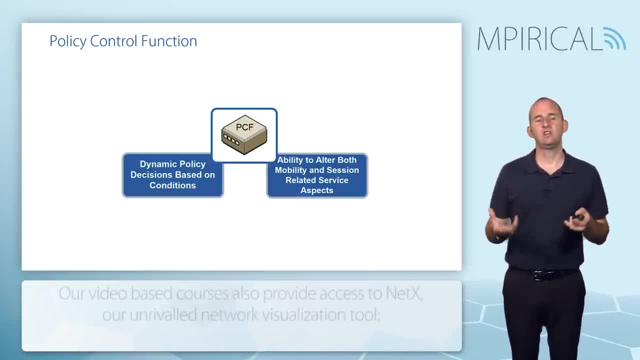 at this present time, are there any network conditions that are going to influence how our subscriber experiences their service? so it might be that the fact the subscribers in a particular geographical location and because they are in that particular cell, for example the PCF, determines that the subscriber needs to be throttled at this time, or 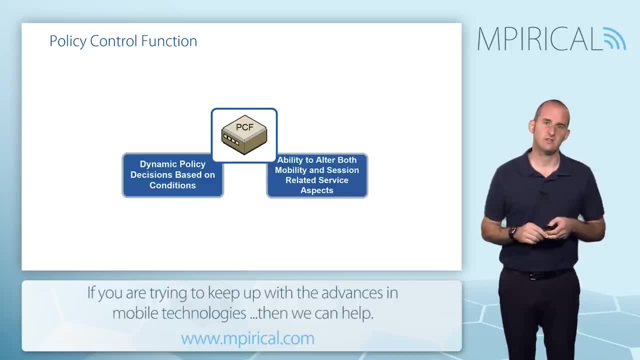 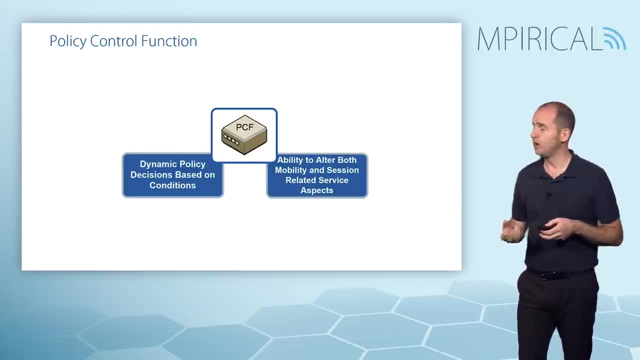 maybe isn't even allowed to get PDU session connectivity. so the PCF, on a dynamic basis, has got the ability to alter both mobility and session related service aspects. so it does play a big part in the overall ecosystem. now notice, when we go back to our main diagram, the PCF does. 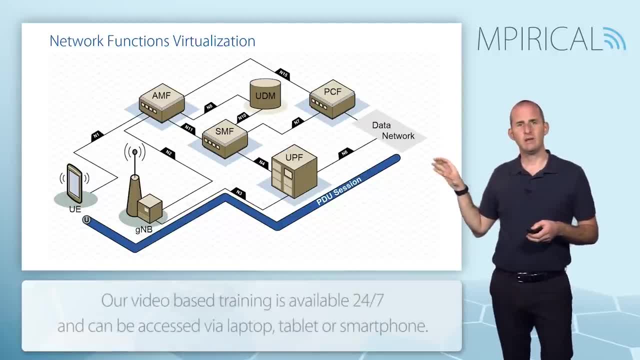 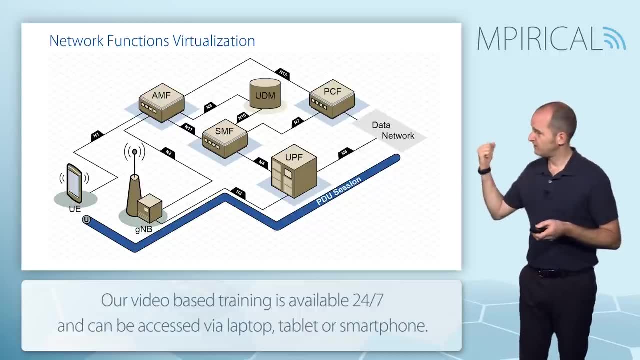 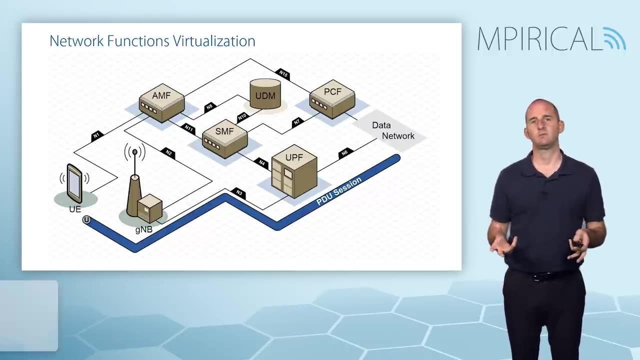 have connectivity into the data network as well, so that PCF can take session related information, such as our subscriber is trying to make a phone call. it can take that information, send it into the 5G call network to ensure that the correct resources are established now. the title of this particular slide is network functions: virtualization. 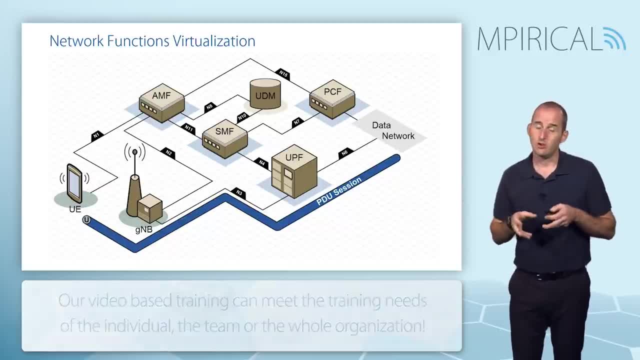 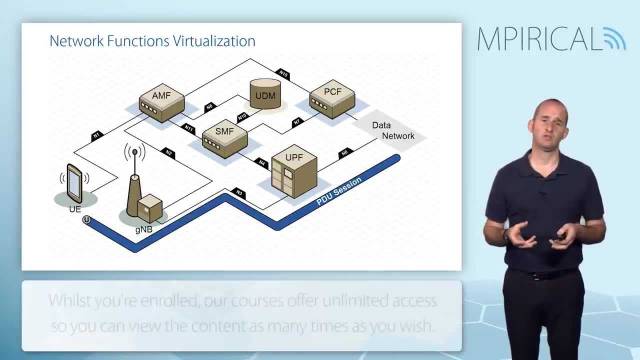 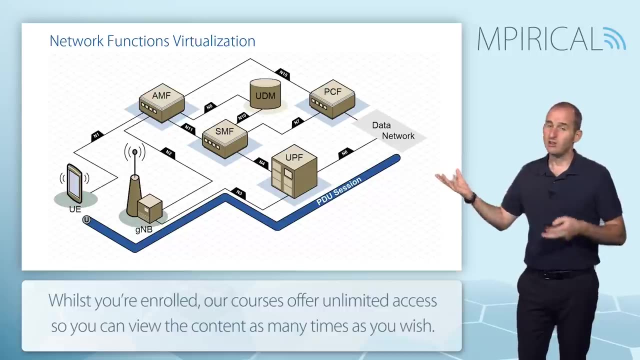 because what is key for our 5G core is that, in reality, much of these nodes will actually be virtualized as part of the NFV infrastructure. now, what do we mean when we say virtualized? well, effectively, these devices that we see are not standalone devices. what they are are software processes. 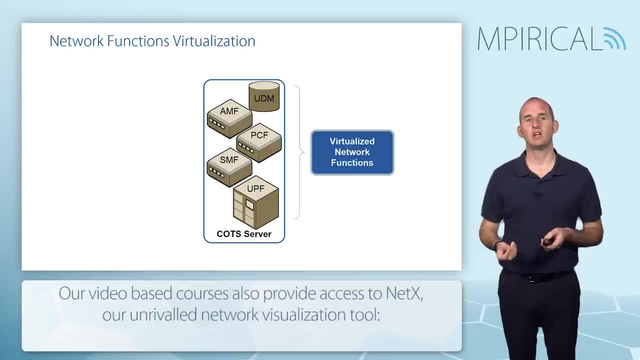 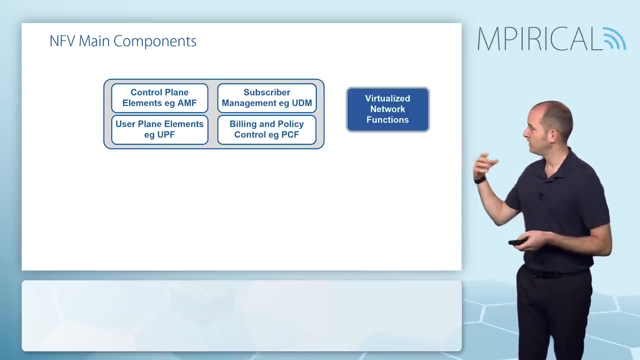 running on what's termed a commercial off-the-shelf server, and this is intrinsically the network functions virtualization architecture whereby we see our virtualized devices, whether it's control plane, potentially user plane, subscriber management, billing and policy control, they can all run as software processes, maybe with a slight exception of the UPF. there's an added 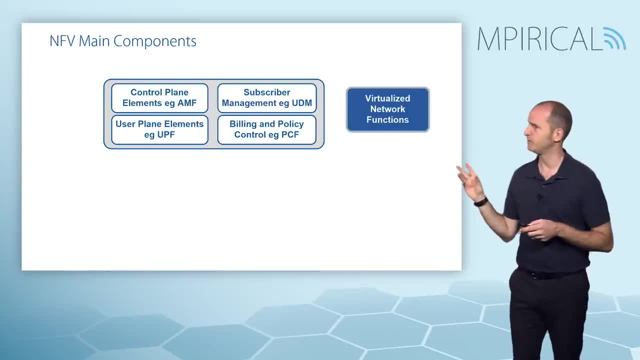 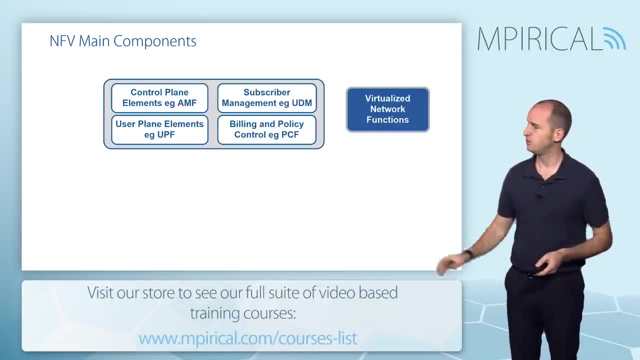 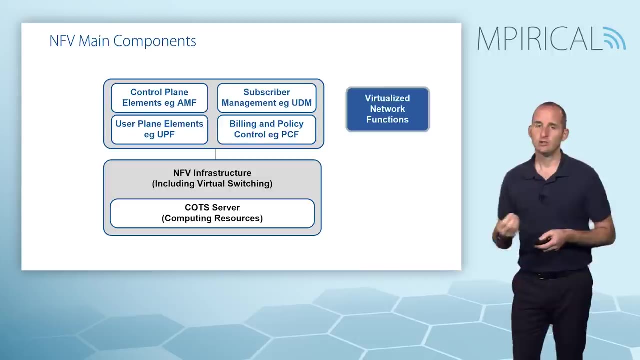 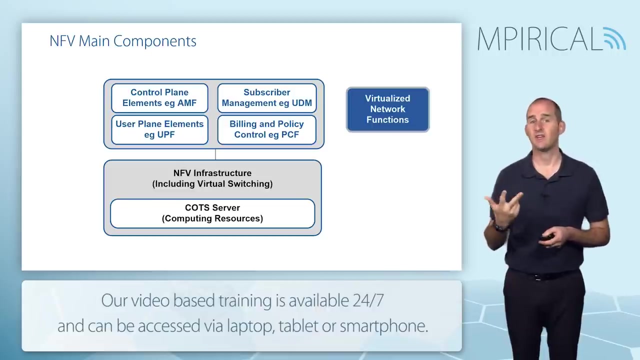 complexity to the user plane, but certainly from a control plane perspective, these elements can run as software processes and the idea behind network functions virtualization is you have a network functions virtualization infrastructure which is fundamentally there to provide these software processes with the compute, the storage and the network resources that they will. 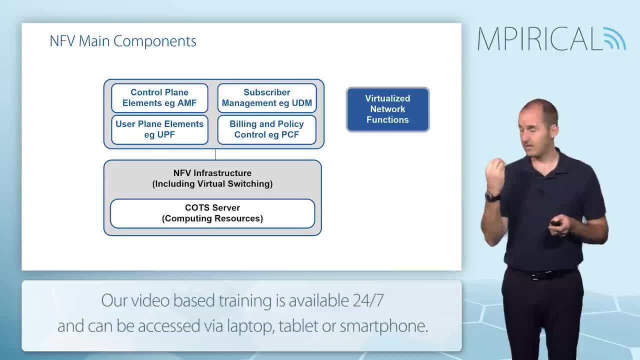 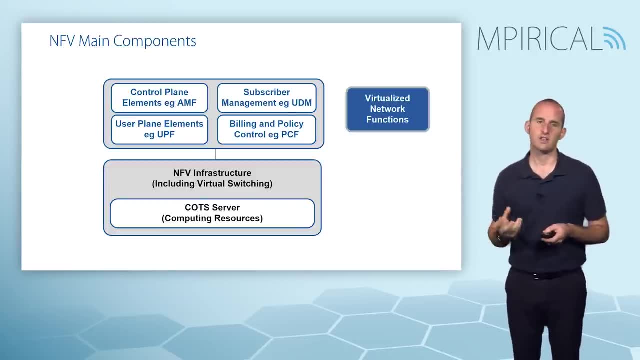 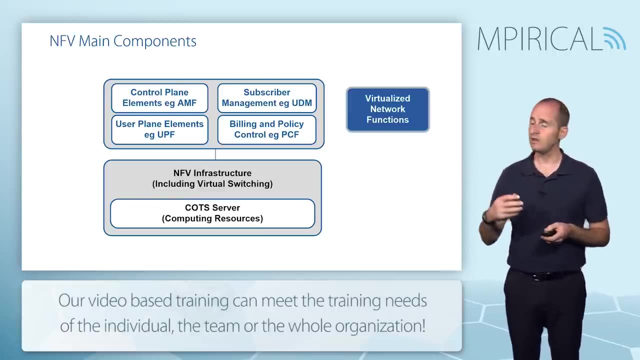 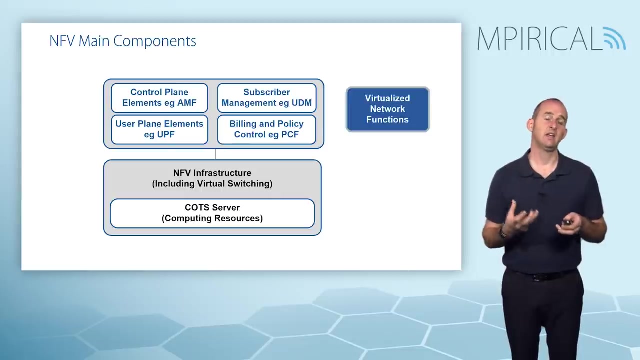 all undoubtedly require. but the key facet is: the NFV infrastructure is a shared infrastructure that all of these software processes will actually use, and it's all built on commercial off-the-shelf hardware. so the cost savings, or the potential cost savings to deploying the core network based on an NFV infrastructure, are 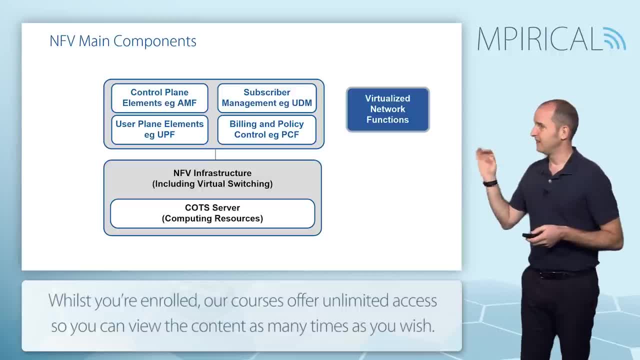 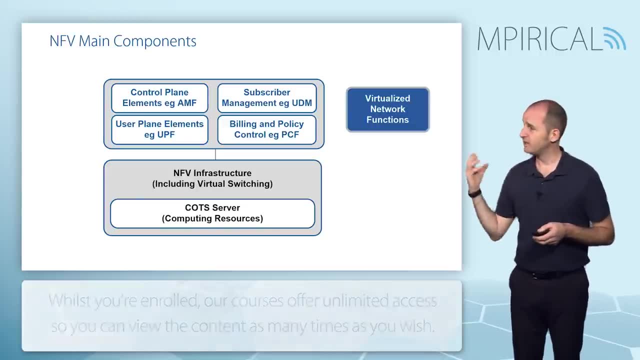 significant now. one of the key benefits of this, other than financial, is the flexibility that you have in your network because these processes are running a software process, and the cost savings that you have in your network because these processes are running a software process is if we need to scale up or scale down capacity. it's much more straightforward. 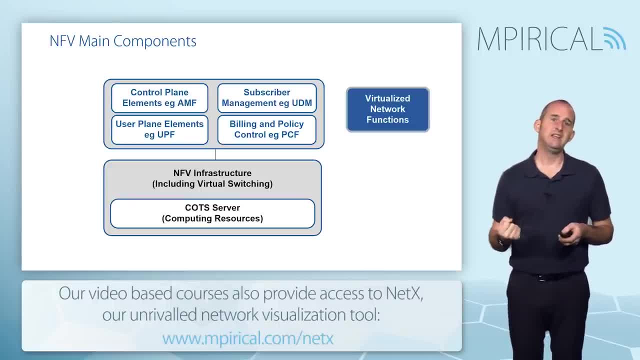 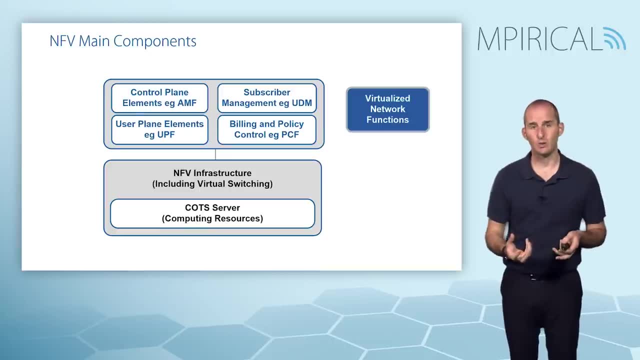 in a virtualized environment. so if we need more AMF capacity, for example, well, if it's a traditional AMF deployed as a piece of hardware, then actually implementing a new AMF in the network can take weeks or even months, whereas if it's a virtualized AMF, well, scaling up capacity could be a matter of minutes. 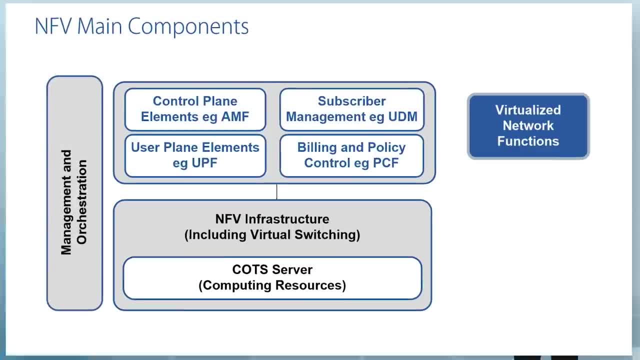 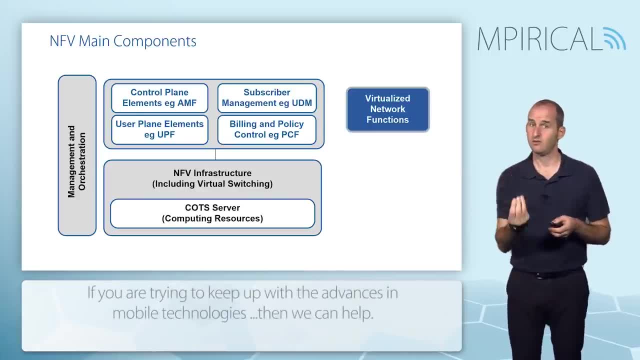 but crucially, you need what's called MANO management and orchestration to facilitate all of this. so this is a piece of the infrastructure in and of itself. so, fundamentally, this is actually what the 5G core will look like. it's a series of virtualized elements, and what's crucial is traditionally where we 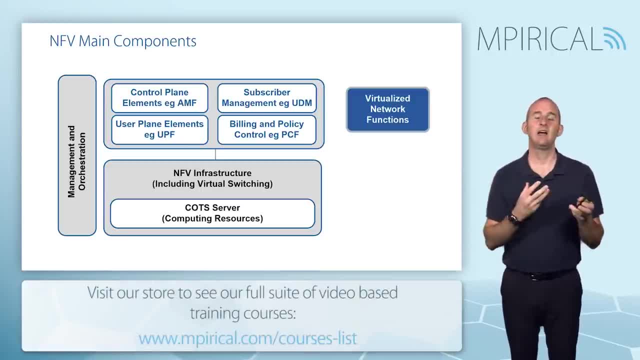 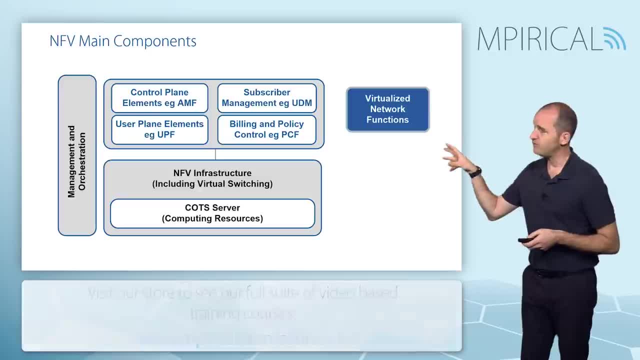 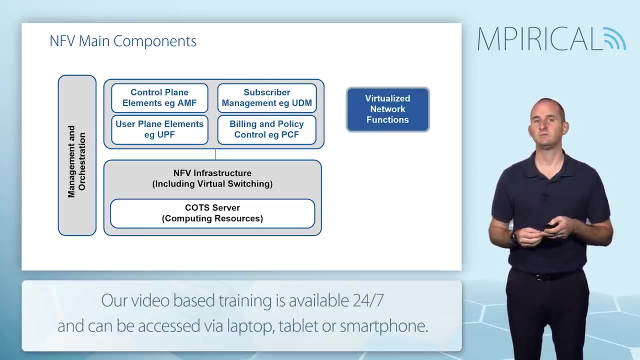 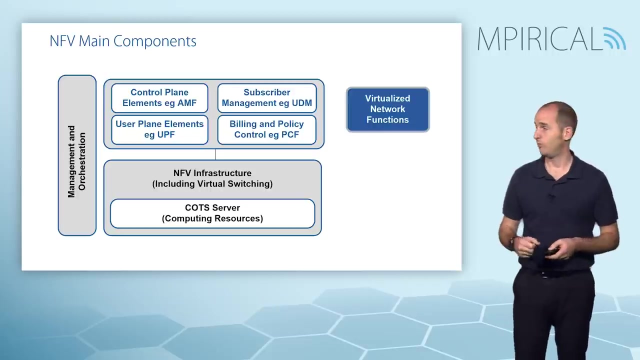 LTE and earlier technologies in 5G. this is all API driven application programming interfaces. these virtualized devices, these virtualized elements are sending API calls to one another in order to communicate. now the final consideration for this session, which is actually closely related, or maybe an enabler for network slicing. so NFV is a 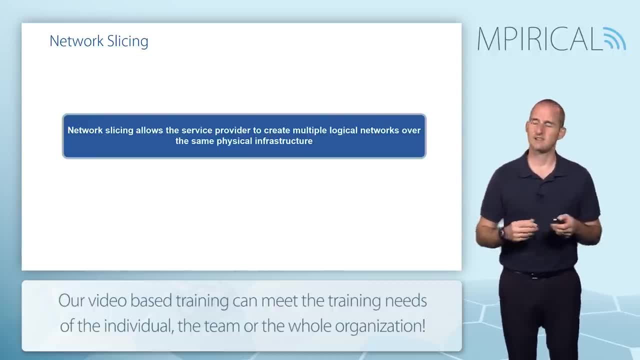 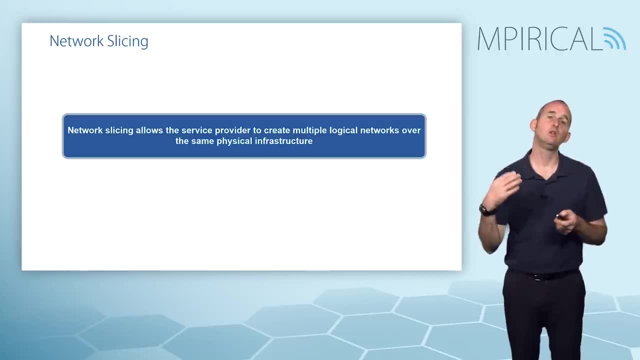 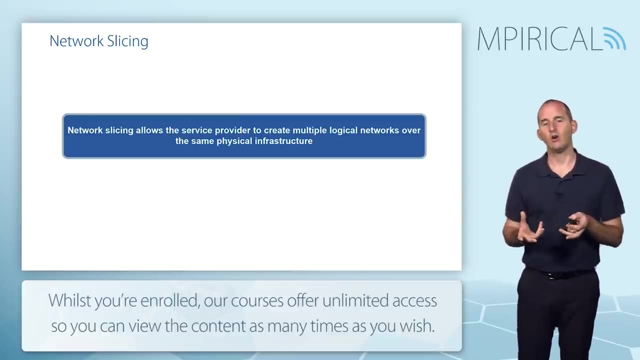 key enabler for this notion of network slicing. but what exactly is network slicing? well, network slicing effectively allows the service provider to create, if you like, logical networks across a common physical infrastructure. now, if you recall, 5g is not just about providing huge data rates to the 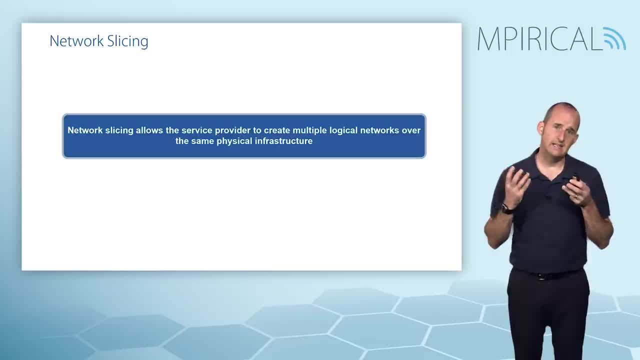 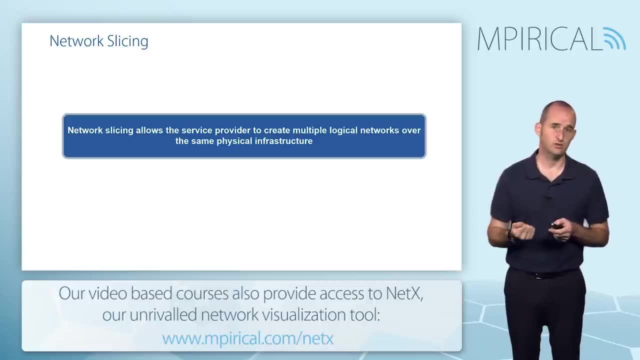 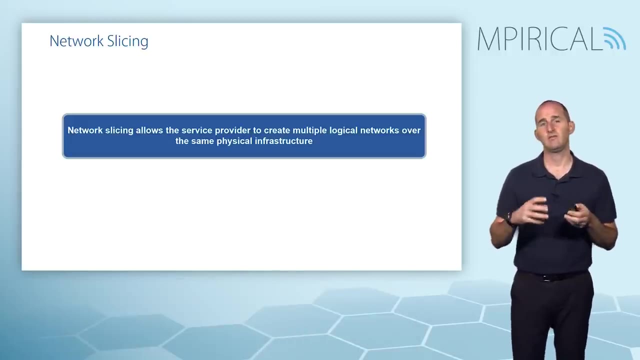 subscriber. 5g is about becoming an enabler network for lots and lots of different applications and lots and lots of different third party users of the network, And the common example is the Internet of Things. So you need to be able to create a very adaptive, flexible network. 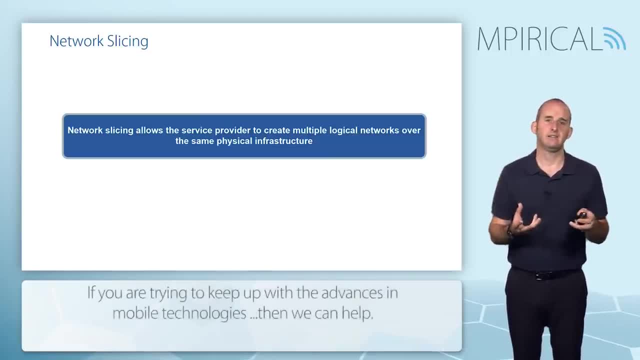 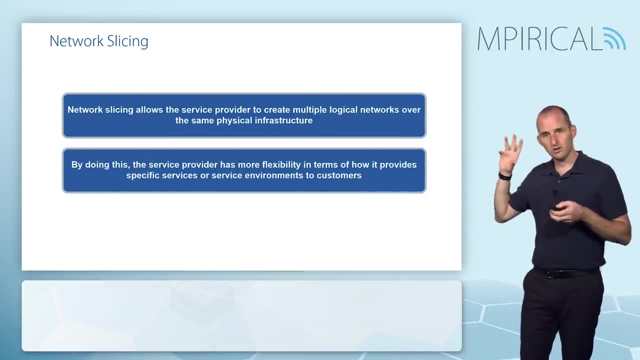 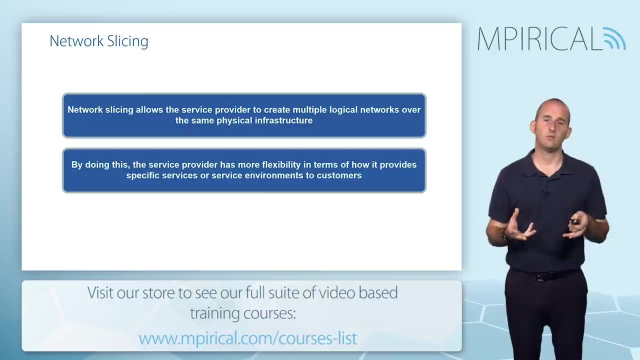 that will provide different customers, different third parties with different features, And network slicing is a perfect solution to do this, because we can create these logical networks across the same 5G physical infrastructure. So we ultimately provide that flexibility to accommodate lots and lots of different potential service environments. 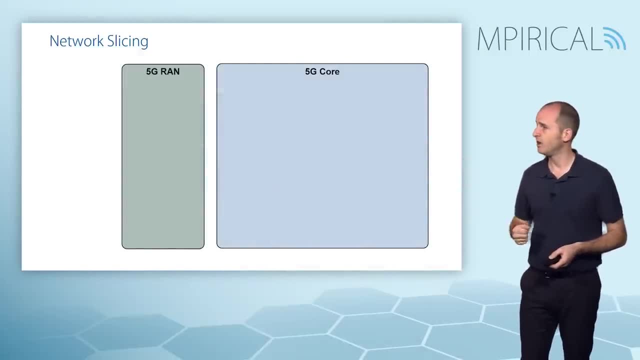 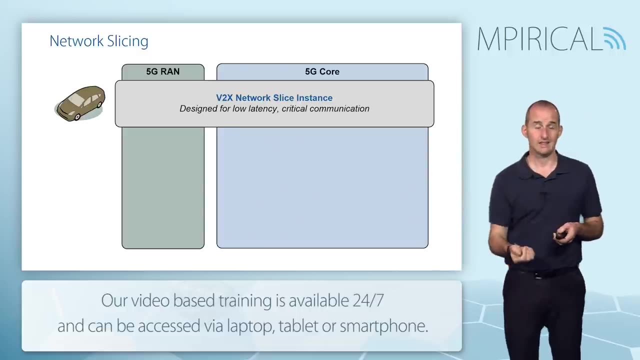 So, to illustrate, there's our 5G RAN and our 5G core network. We might have, for example, a V2X network slice And clearly the characteristics of V2X are low latency, critical communication, Now on top of the same physical infrastructure. 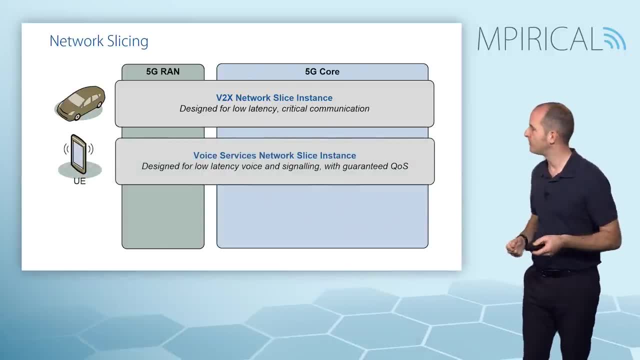 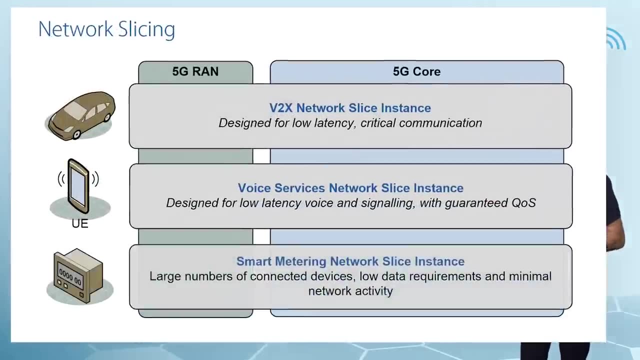 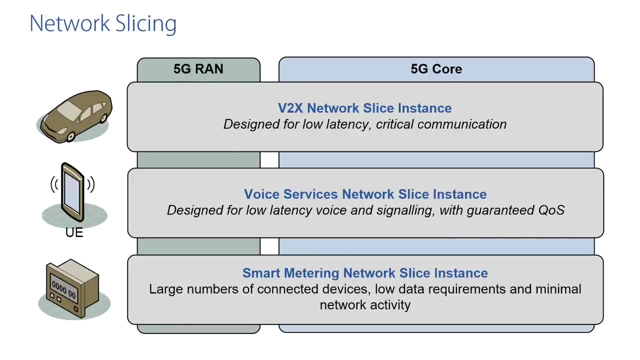 we could have voice services for our typical human subscribers. We need low latency for our voice and signalling and we need guaranteed quality of service. And finally, we might have some kind of smart metering network slice where we need to accommodate large numbers of connected devices. 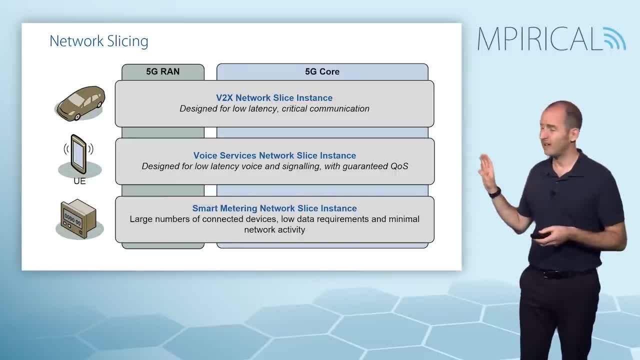 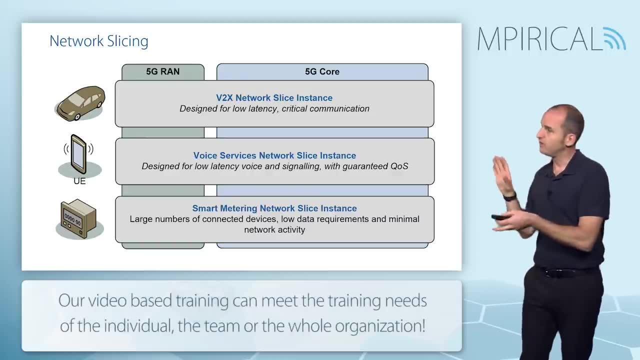 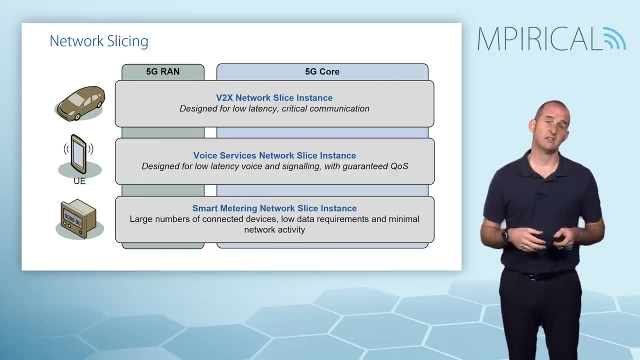 but they have actually fairly low data requirements and relatively minimal network connectivity and activity. potentially So lots and lots of different environments here that can be accommodated by network slicing And, in terms of the standards, in actual fact an individual device is able to connect. 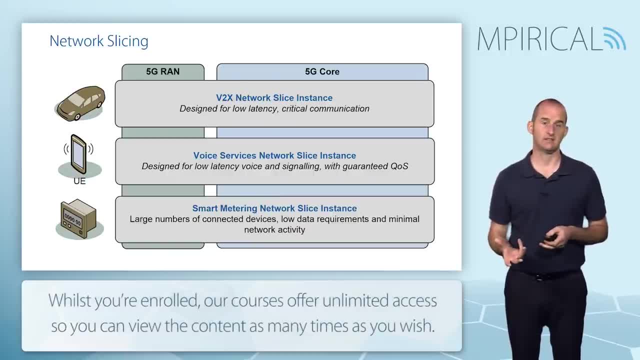 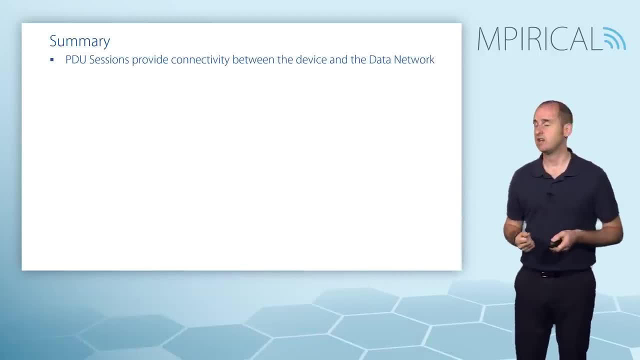 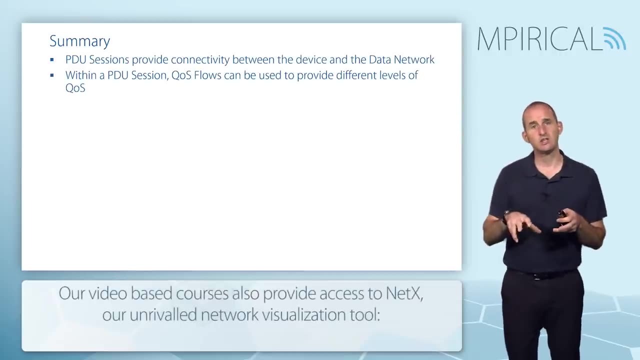 to up to eight network slices simultaneously. So, in summary then, we talked to begin with about PDU sessions, and we saw that they provide connectivity between the device and the data network Within a PDU session. we have QoS floors and they are designed.